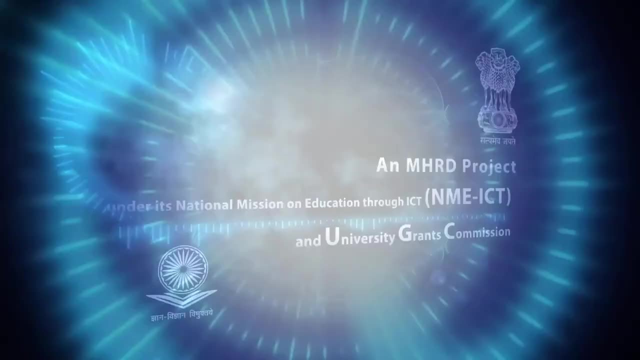 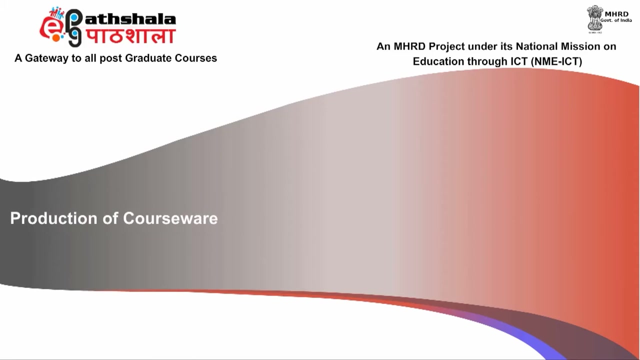 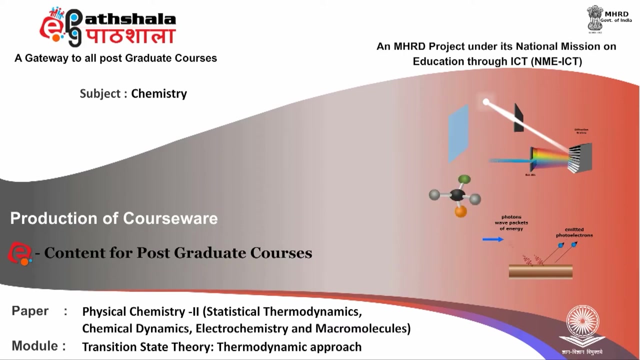 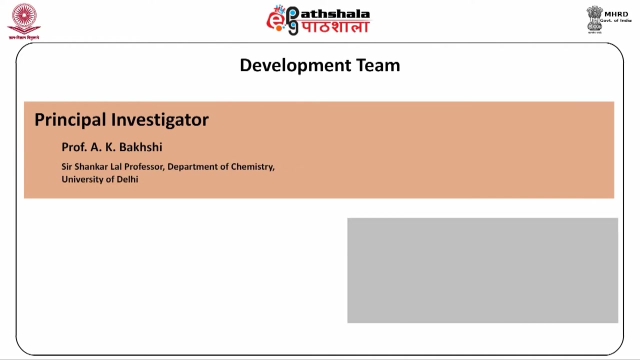 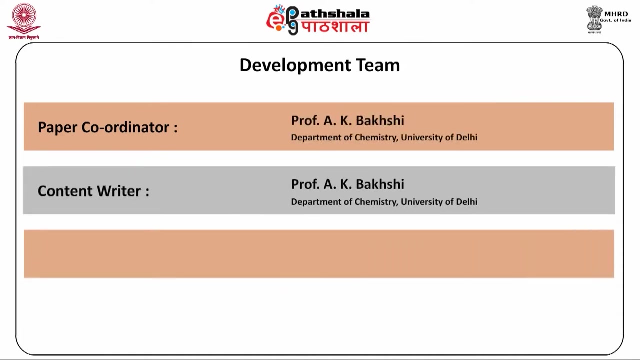 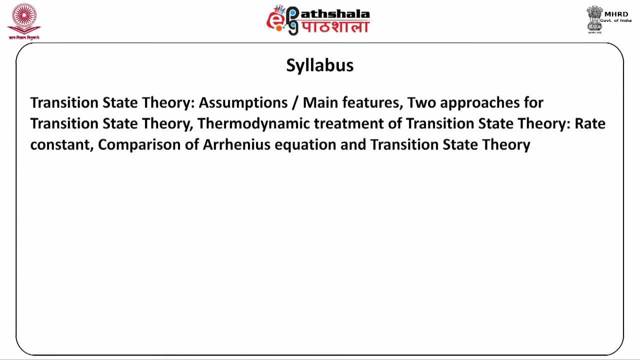 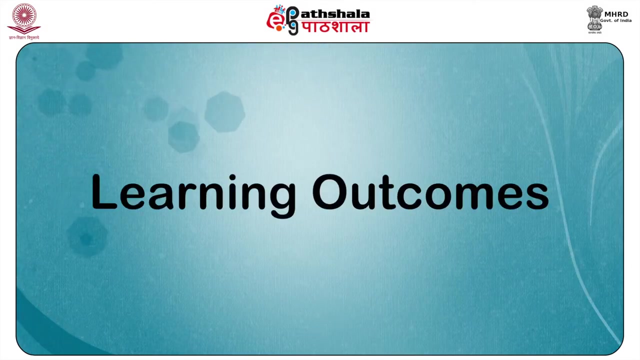 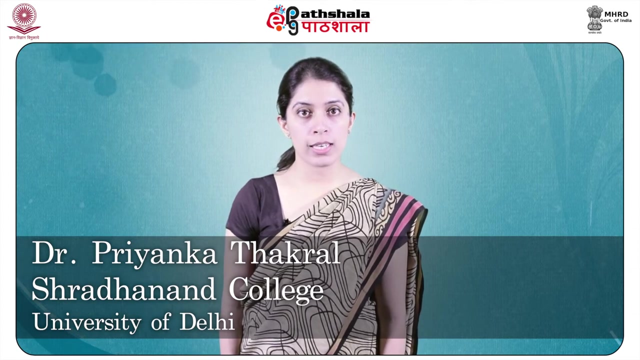 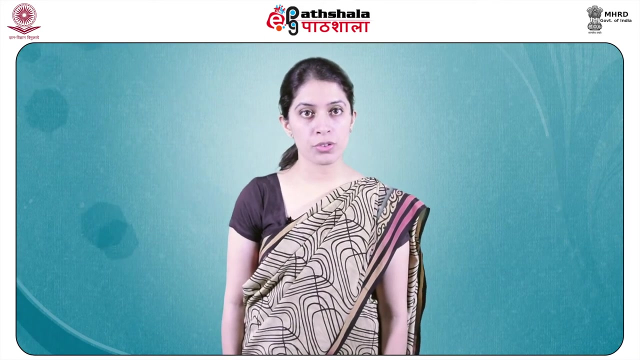 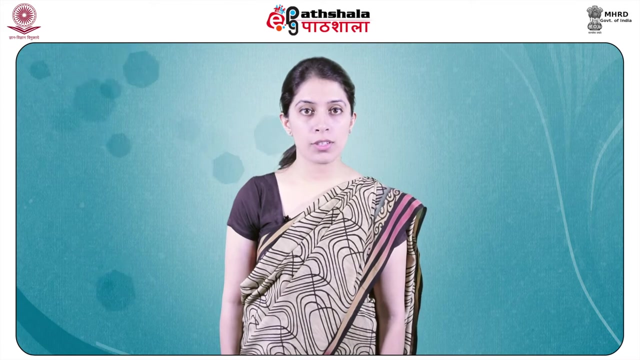 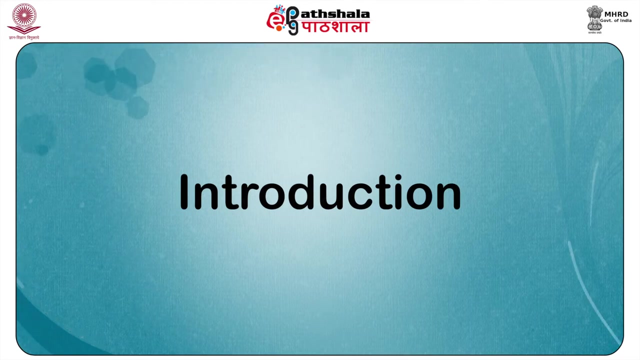 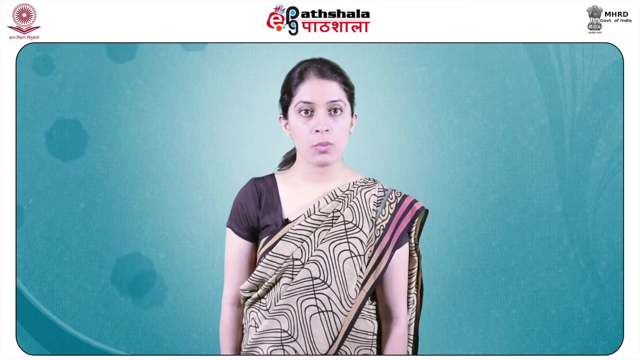 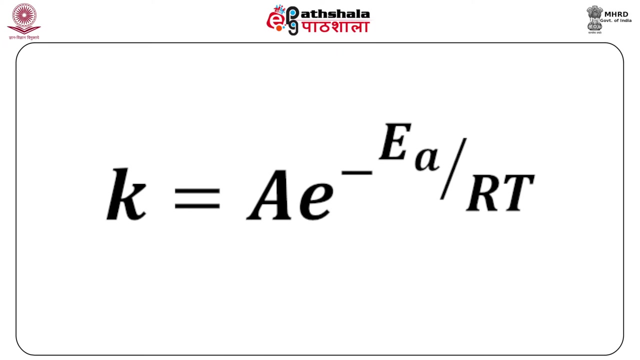 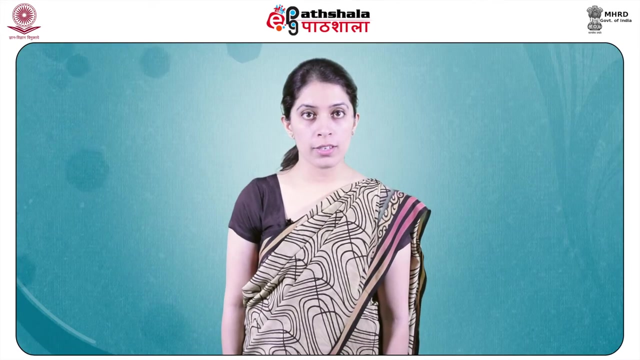 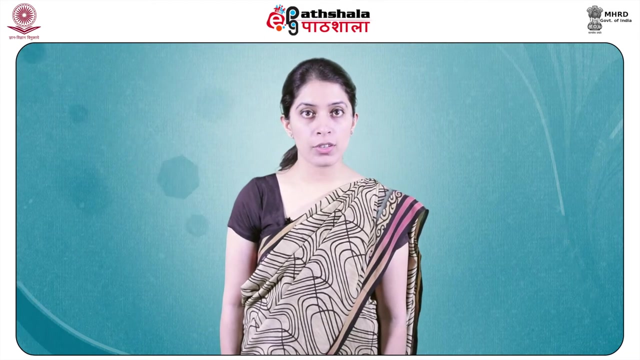 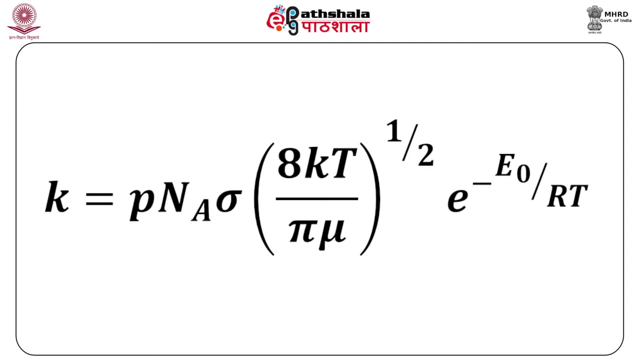 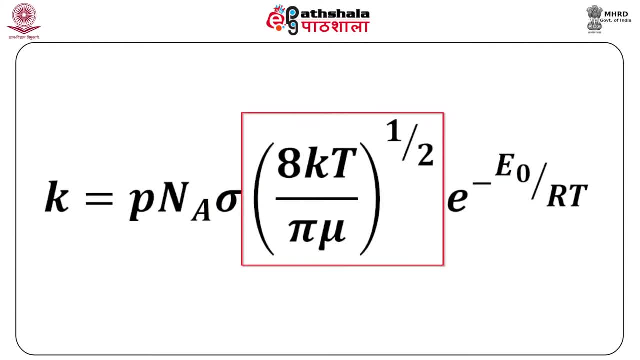 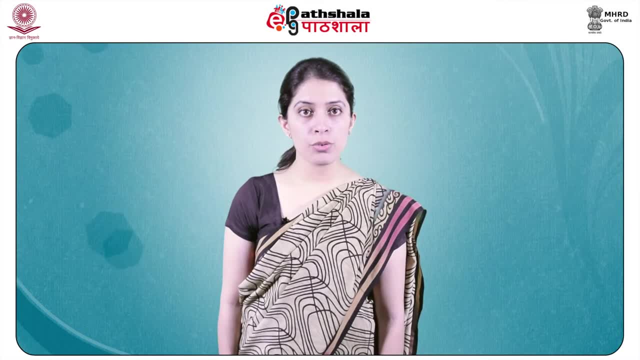 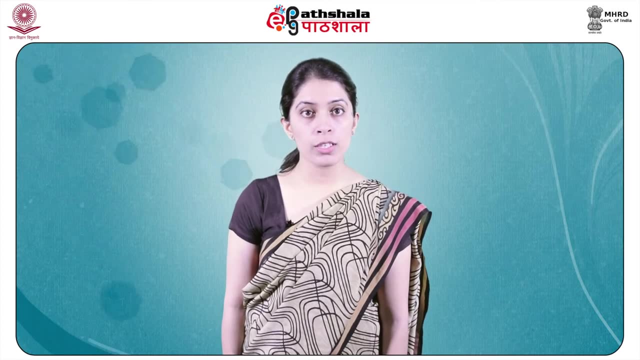 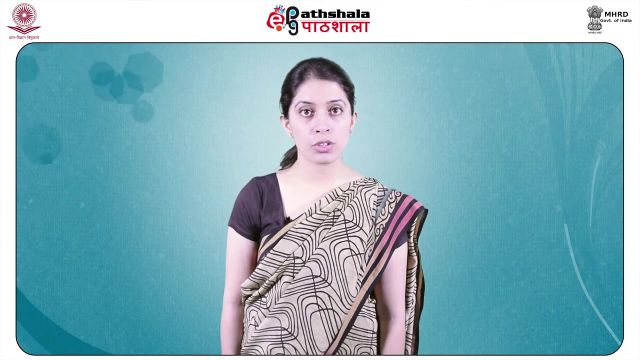 e0 is the energy barrier and the under root term refers to the average velocity of the molecule and p refers to the steric factor. The major drawback of collision theory is the difficulty in calculating the steric factor from molecular geometry for complex molecules. So in this module we will discuss another important theory for determination of rate constant, that is, transition state theory. 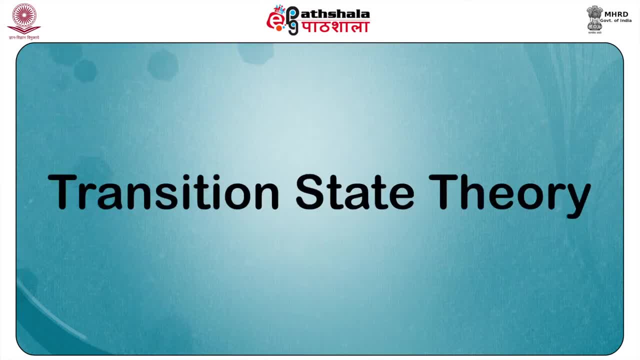 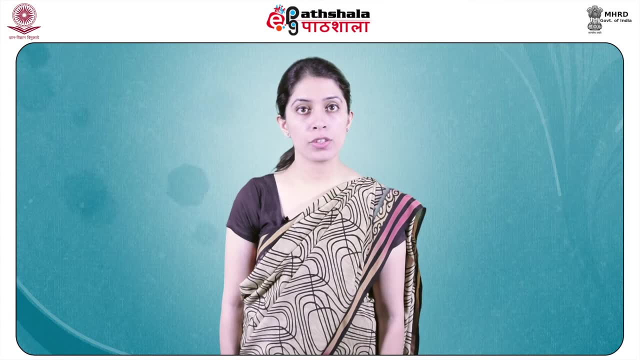 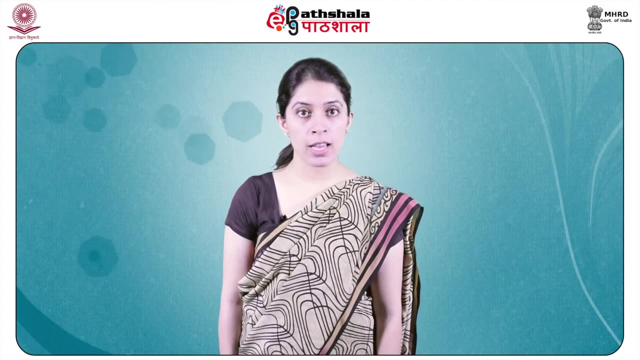 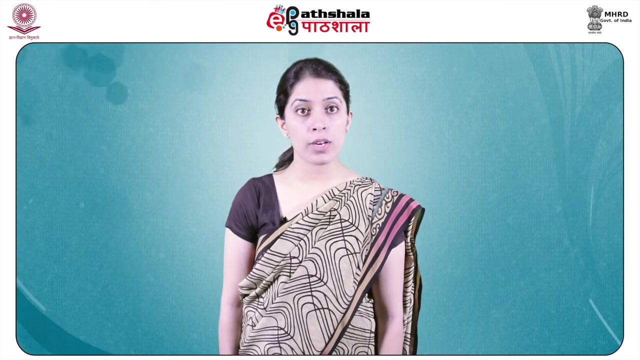 Now let us discuss transition state theory. Transition state theory is popularly referred to as activated complex theory or theory of absolute reaction rate. This theory was developed in 1935 and is an attempt to express rate constant in terms of a model of sequences or episodes that take place during the reaction. 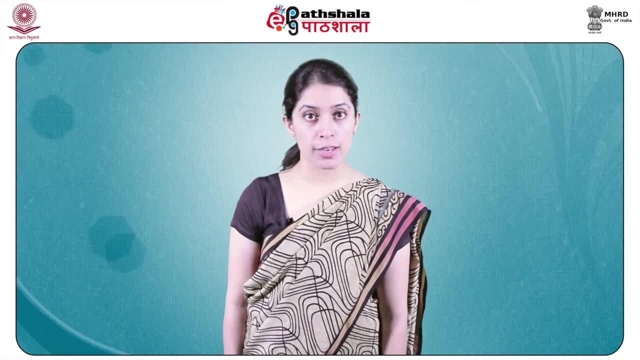 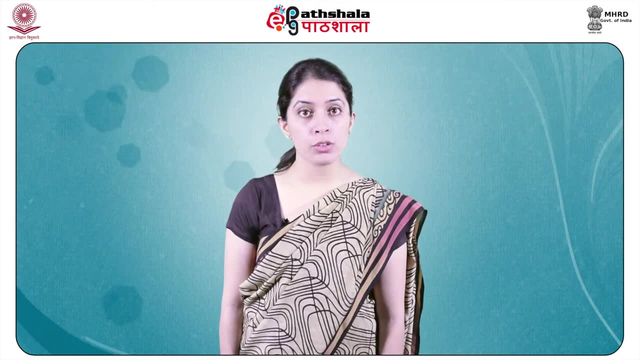 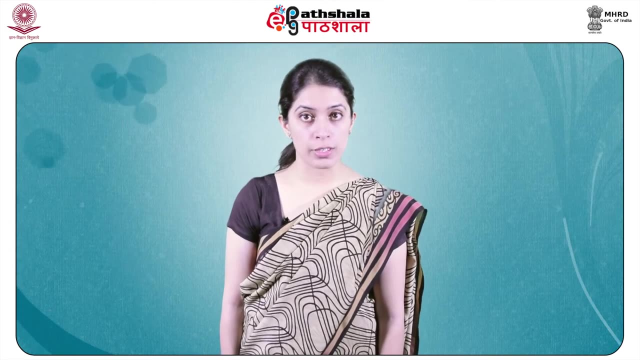 This theory is applicable Essentially to gaseous reactions, and the advantage of transition state approach is that the quantity corresponding to steric factor appears automatically in the rate constant expression, which was a drawback in collision theory. The transition state theory depicts the formation of transition state complex, which is also sometimes referred to as activated complex, which is formed from the reaction between reactants A and B. 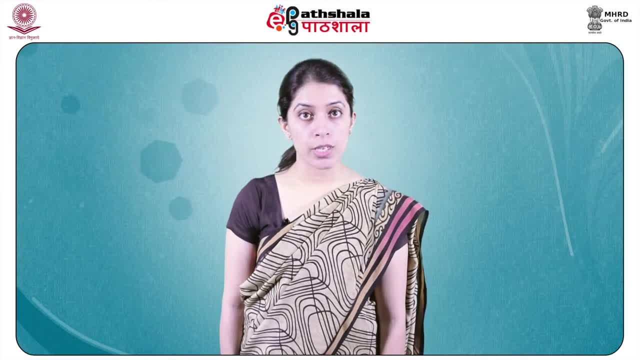 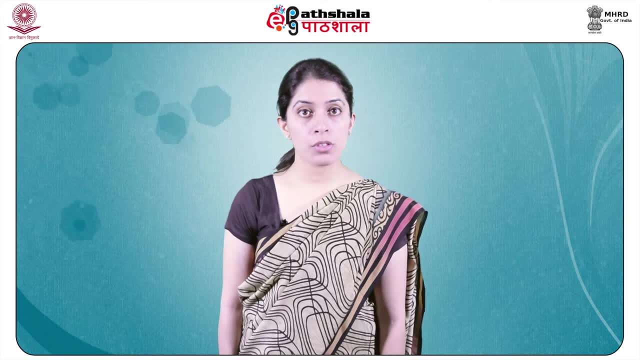 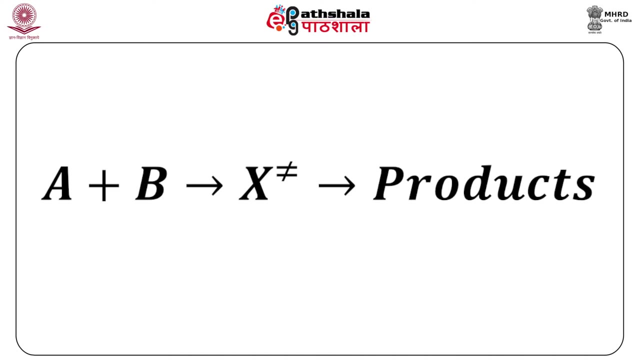 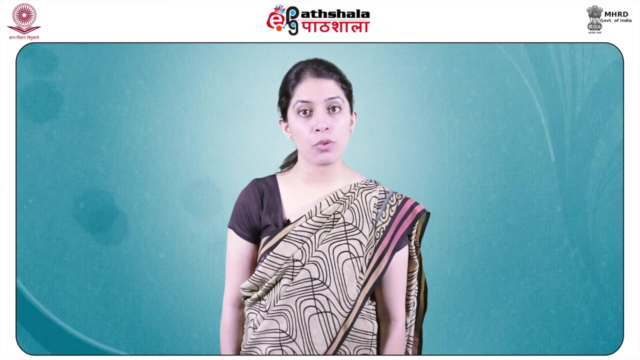 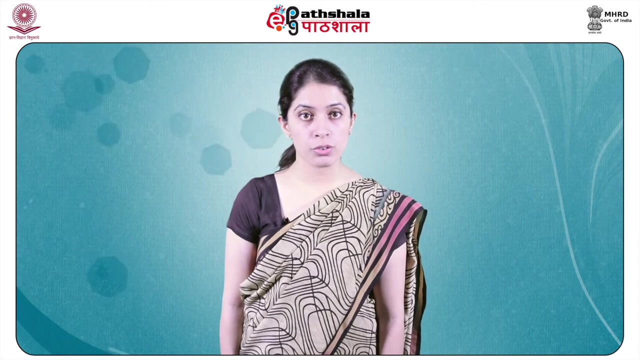 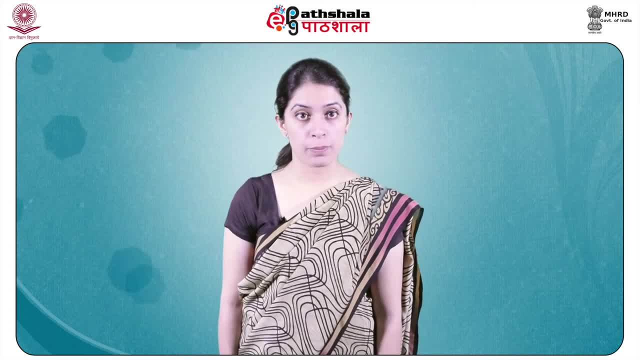 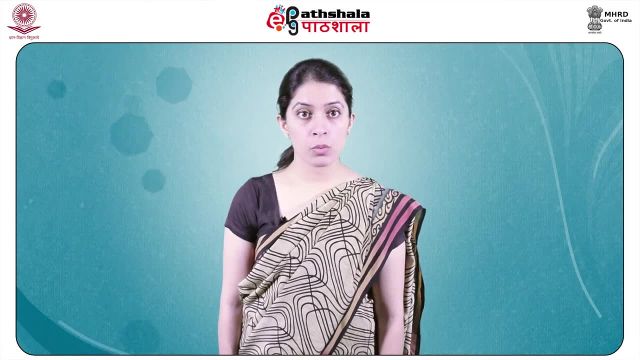 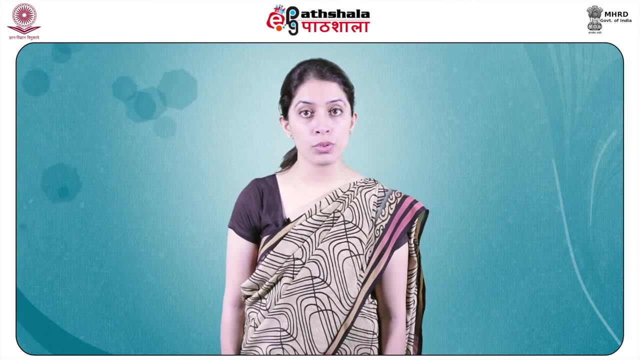 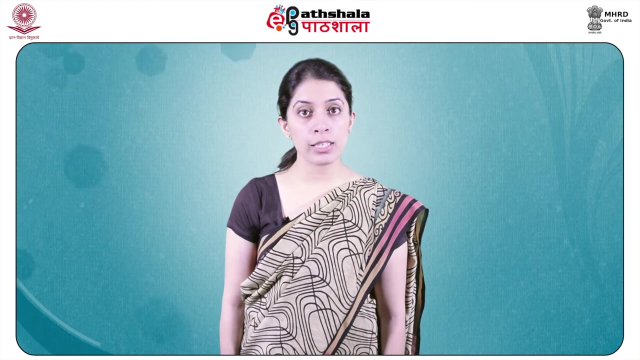 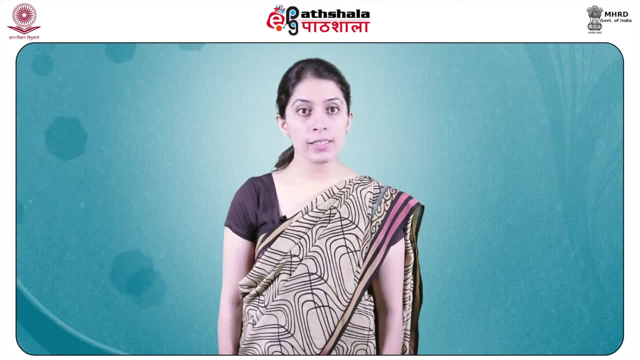 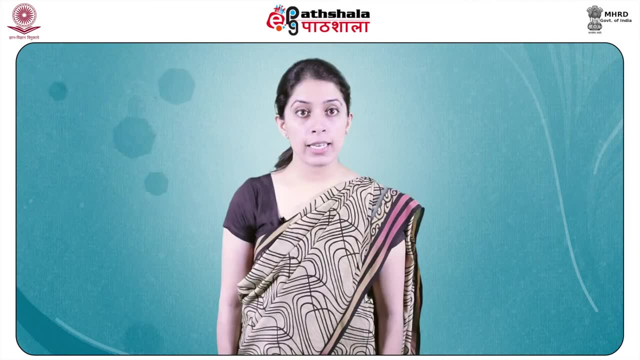 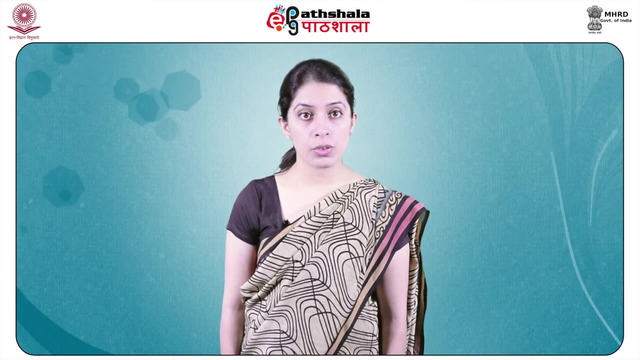 term in context of this theory. Let us now look at the main features of transition state theory. It is assumed that a transition state complex is in equilibrium with the reactants and that the rate at which the transition state complex decomposes to product, which is a slower 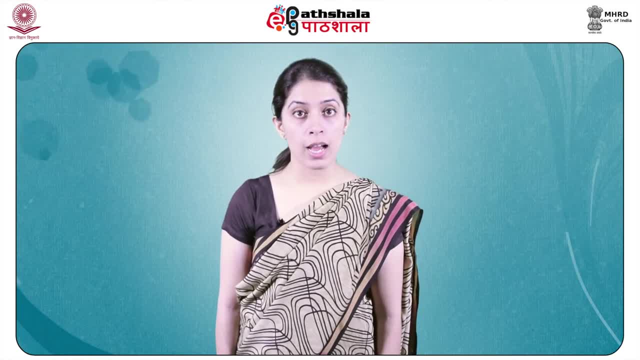 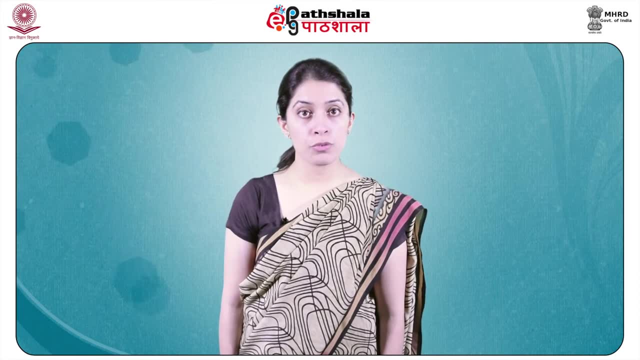 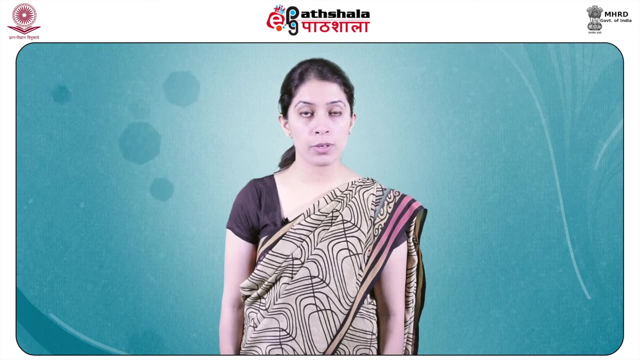 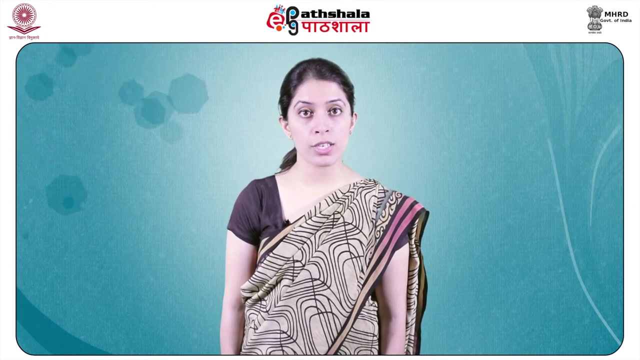 rate determining step depends on the rate at which it passes through the transition state. The major assumptions of this theory are: collisions are responsible for a chemical reaction and it is important to know that this equilibrium is not the conventional equilibrium that we talk about. Thirdly, the reaction coordinate describing the conversion of transition state complex to product can be mapped onto a single degree of freedom of transition state complex. If product formation involves breaking of a bond, let us say for a diatomic molecule, then the vibrational degree of freedom corresponding to bond stretching is taken as reaction coordinate. Now let us now assume the following bimolecular reaction: 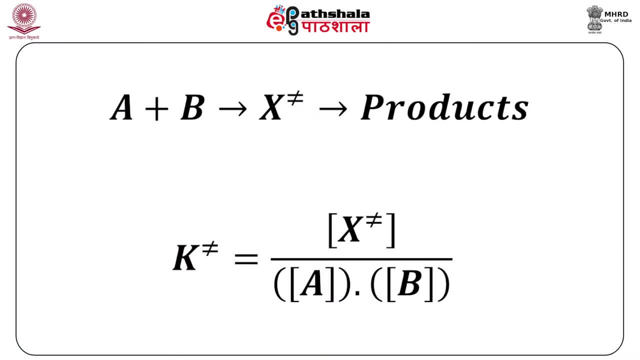 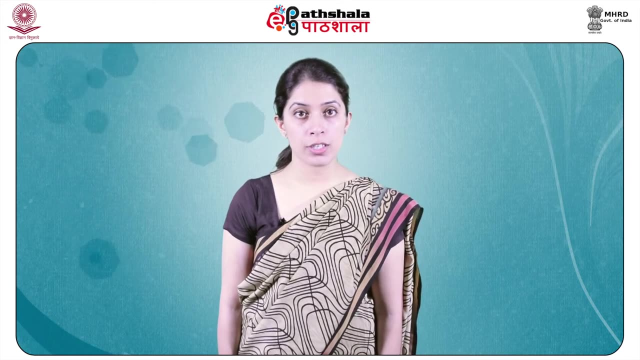 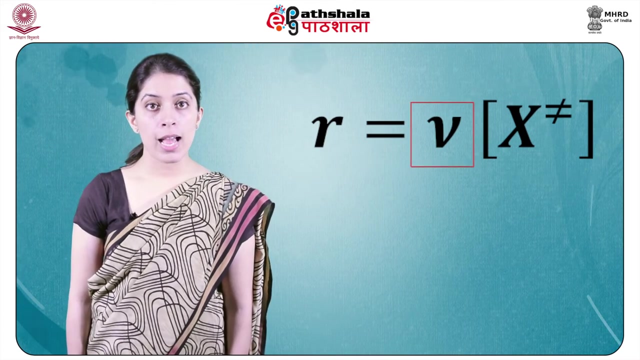 A plus B, giving transition state complex, which gives products. The equilibrium constant for this reaction is as follows: K is equals to concentration of transition state complex upon product of the reactants and the rate as per transition state theory depends on 2 factors: firstly, concentration of the transition state complex and secondly, 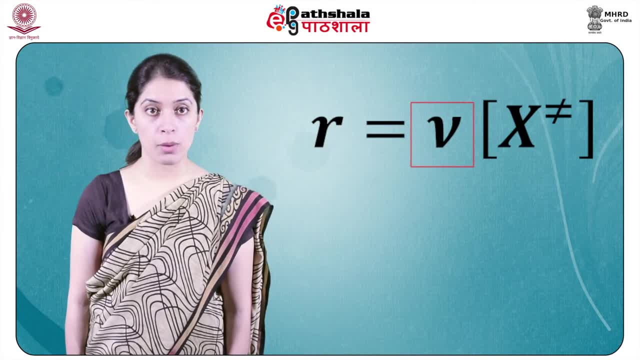 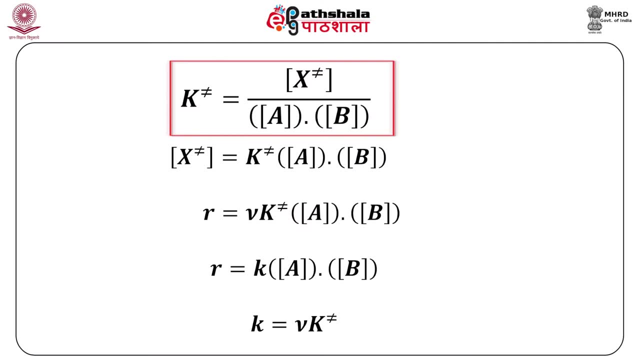 the frequency of decomposition of activated complex. So rate becomes frequency into concentration of activated complex. Now if we consider the equation for equilibrium constant and we rearrange that to obtain the concentration of the activated complex, we get K concentration of A concentration of P. Now if we forced a sleep, 那我们有一种突升段, and then we rearrange, stop over. there and the rate will be bewildering above so rate will earn a Ç Forροять기� flashup of this charge. we do the same thing as we did the phase first time. so rate becomes frequency of active complex and thenquanten�in tiуatt within the levels we get Xi※. 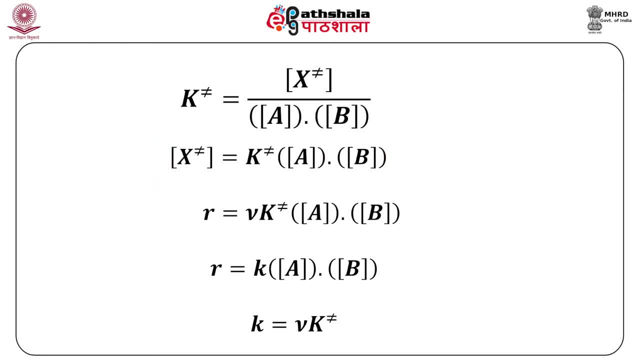 concentration of A, we get P fís commerce. We now get rA※ as א※ iemand zu eqquilibrium時候? of activated complex. So we leave the field of fire frequency and we are going to get Now, if we substitute the concentration for activated complex so obtained using the equilibrium, 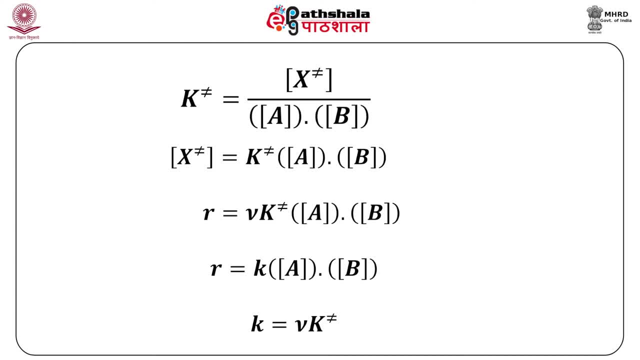 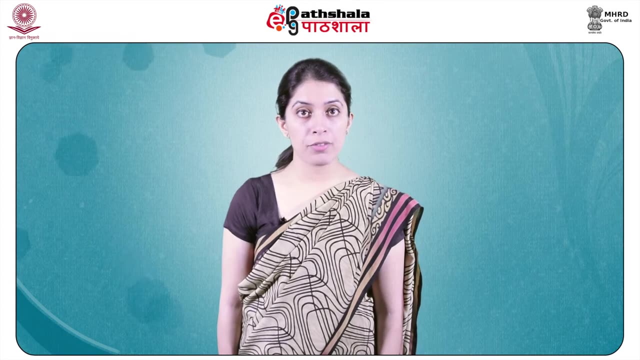 constant equation. we get the rate as frequency into K, into concentration A, into concentration B, or simply we can write the equation as: R equals to K, into A, into B, as shown Now. in order to derive the expression for rate constant, there are two different approaches under transition state. 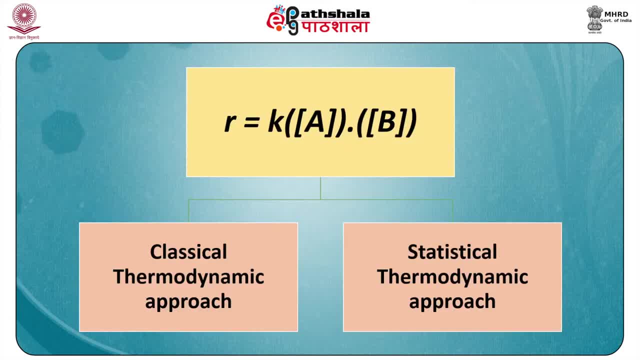 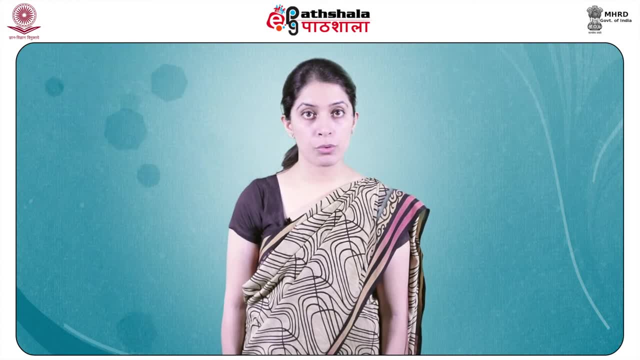 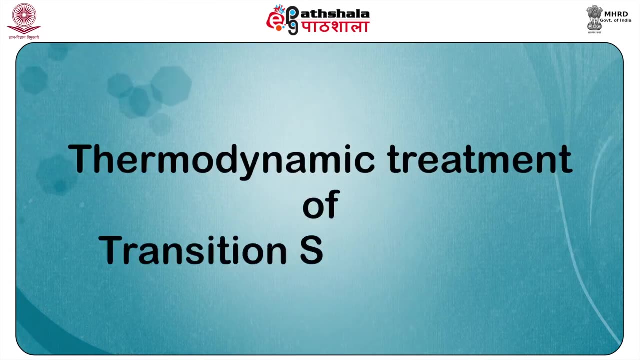 theory. One is the classical thermodynamic approach and the second is statistical thermodynamic approach. In this module we will take up the classical thermodynamic approach first and the statistical thermodynamic approach will be taken up in the next module. Thermodynamic treatment of transition state theory. Let us consider a reaction as shown: Bromine with hydrogen molecule. 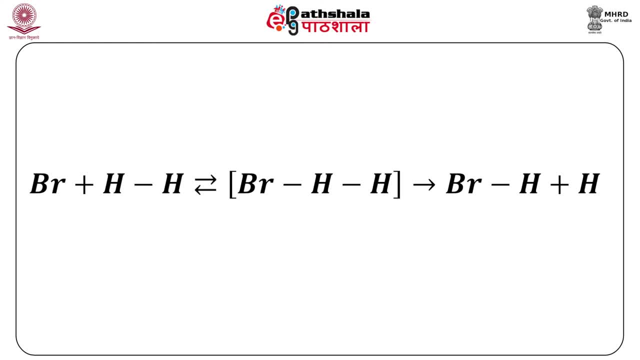 so there is a bond between two hydrogen atoms and the transition state complex is shown in the following manner: bromine attached to hydrogen, which is further attached to hydrogen, and this gives the product as bromine reacting with hydrogen molecule where there is a single bond between two. 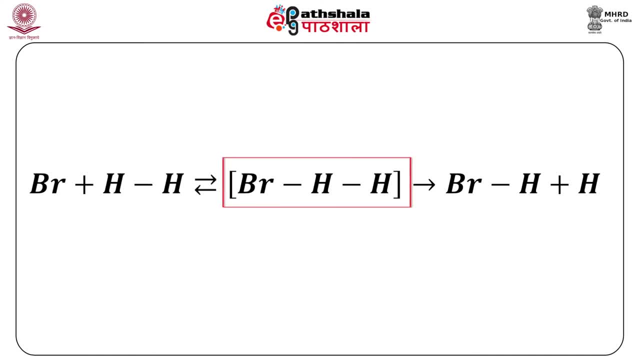 hydrogen atoms. Now this gives the transition state complex, as bromine attached to hydrogen, which is further attached to hydrogen. This transition state complex gives the product as a bond formation. Now let us consider a reaction between hydrogen and bromine and a hydrogen atom. This reaction proceeds. 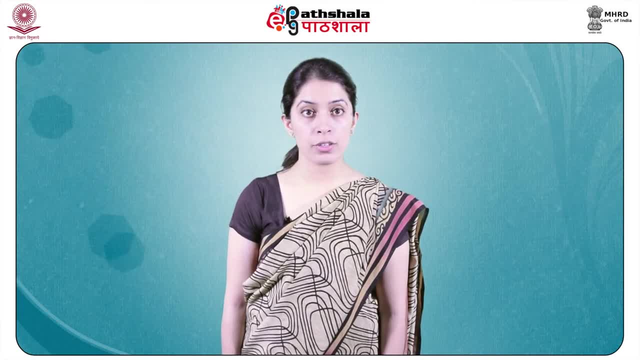 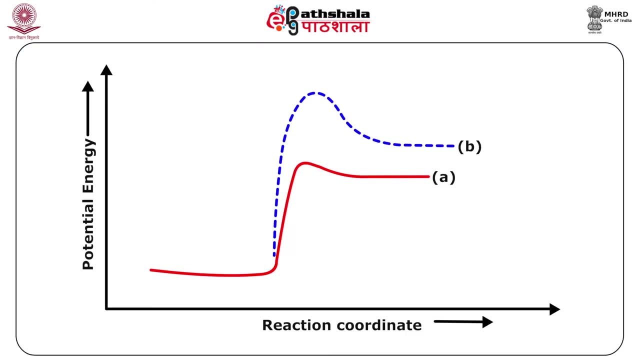 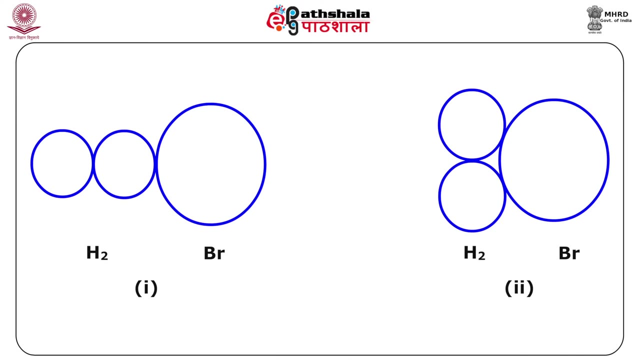 through a transition state which has higher energy than that of the reactants and products, and this reaction sequence is shown in the, where on the y-axis we have potential energy and on the x-axis we have reaction coordinate. Now, very firstly, one can notice that the collision between 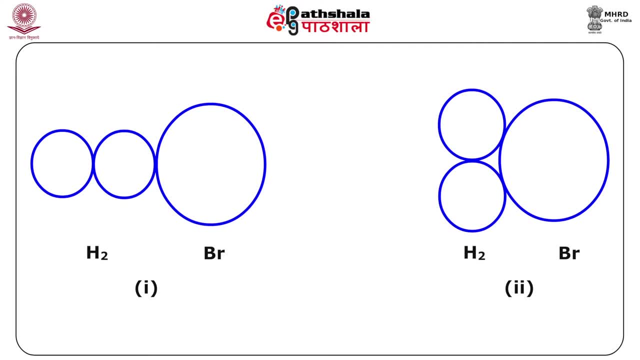 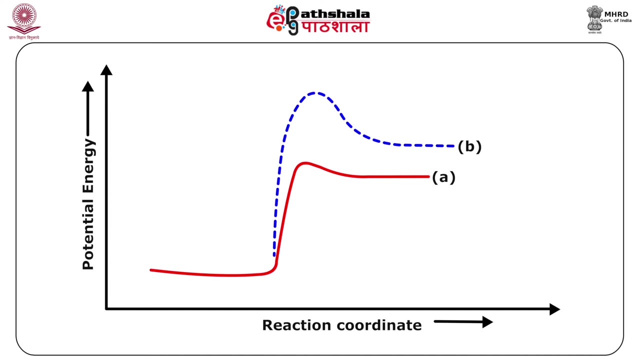 bromine and hydrogen can occur in two possible ways, That is, one is sideways collision and the other is head on collision. as shown in the figure Now, the side on collision is presented by curve A and the head on collision is represented by curve B, and one can see that the transition state for side on collision is lower in energy in comparison to. 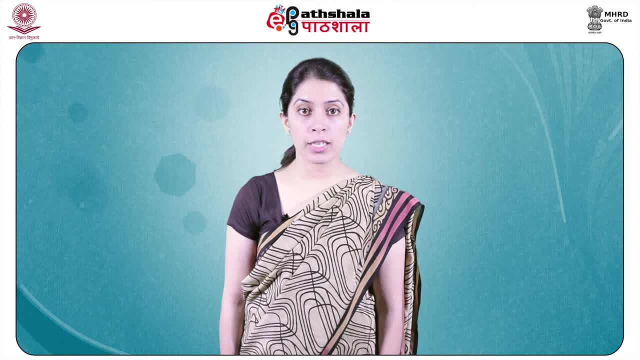 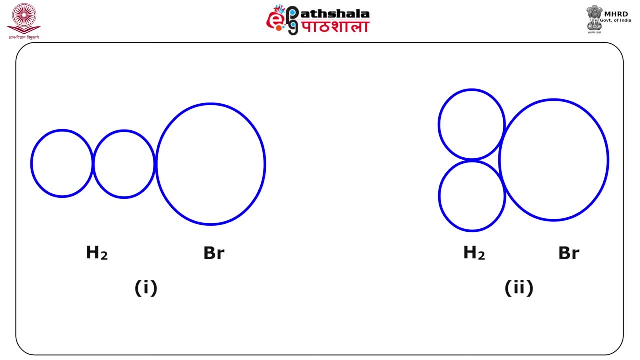 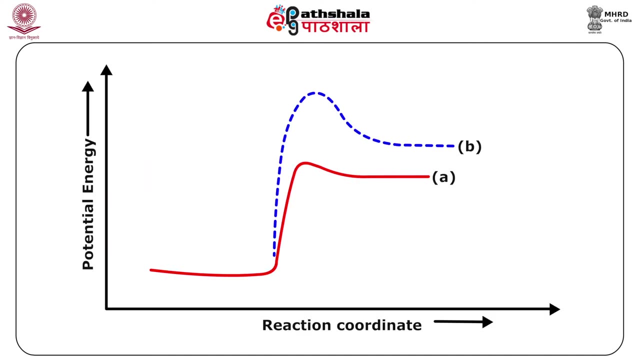 head on collision. In order to understand this graphical plot of potential energy as a function of reaction, it is important to note that the collision between bromine and hydrogen can occur in two ways, as shown Now in the potential energy plot. curve A corresponds to the way of collision, as 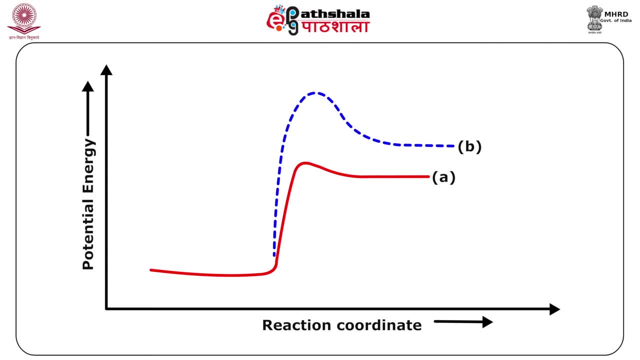 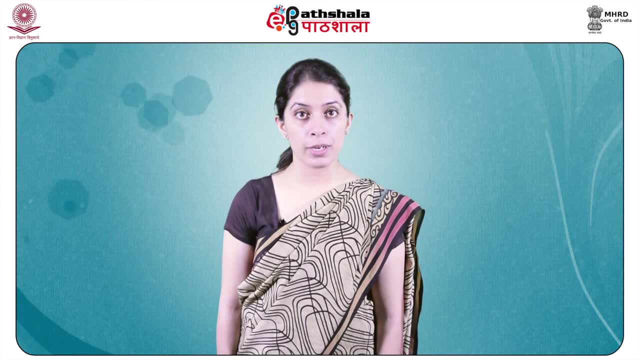 shown in the figure 1, and curve B gives the potential energy plot for the collision shown in figure 2.. The transition state theory predicts the formation of a transition state complex as represented for this reaction as bromine attached to hydrogen which is attached to hydrogen. 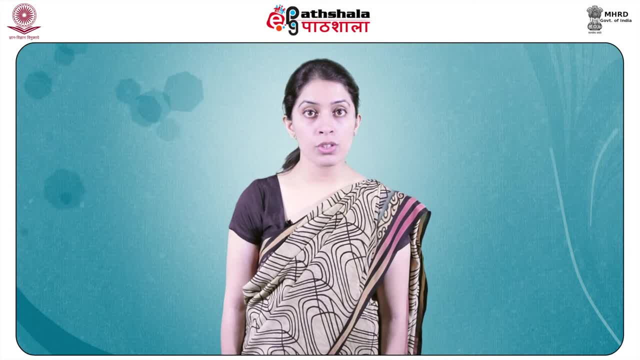 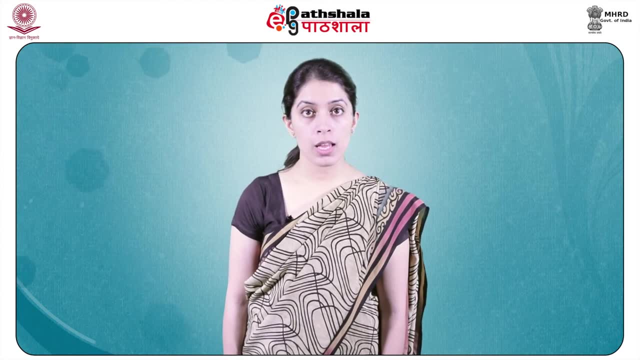 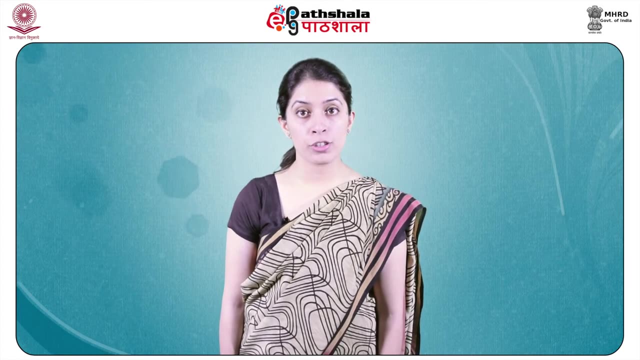 It is important to note over here that this transition state complex is not an intermediate compound. It is a molecule in the process of breaking or forming bonds. This transition state complex is not stable and is present at maximum in the potential energy curve, as shown. 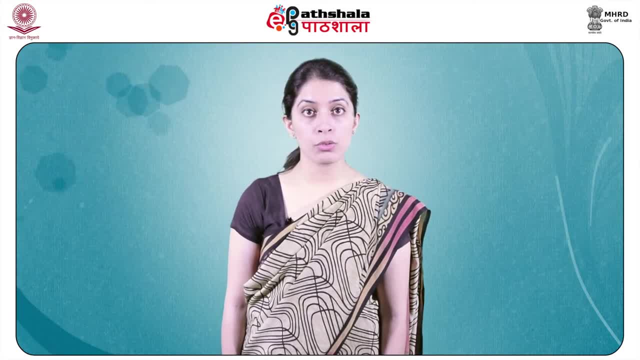 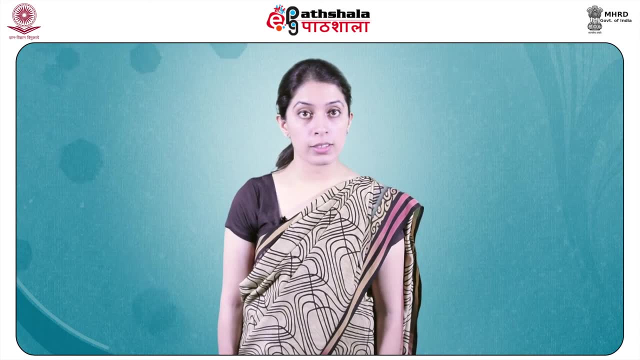 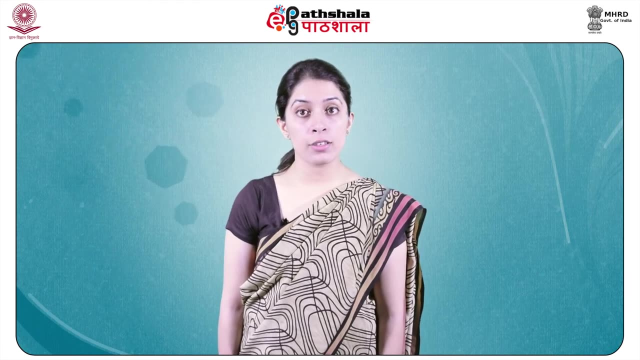 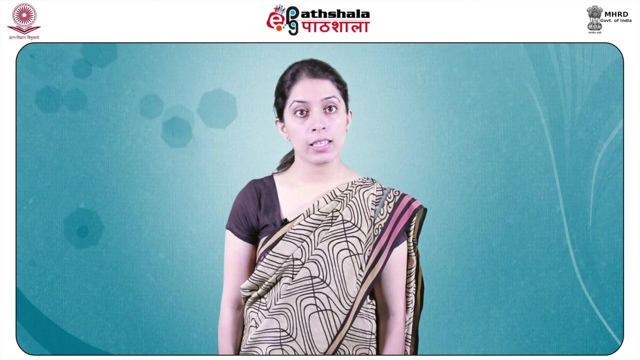 This maximum point of the curve corresponding to the transition state complex is called the saddle point. Further, one needs to know that that this bond breaking is an energy demanding process and the bond making is an energy releasing process. The net energy requirement for the formation of transition state complex and the 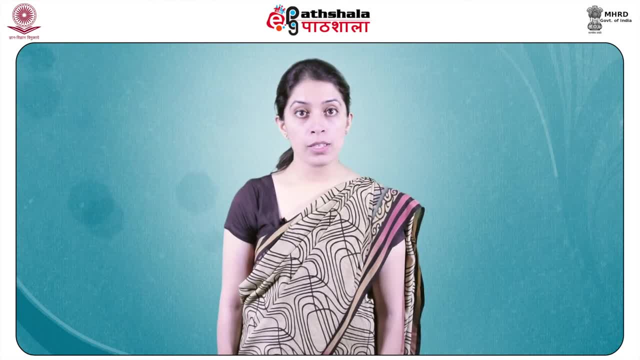 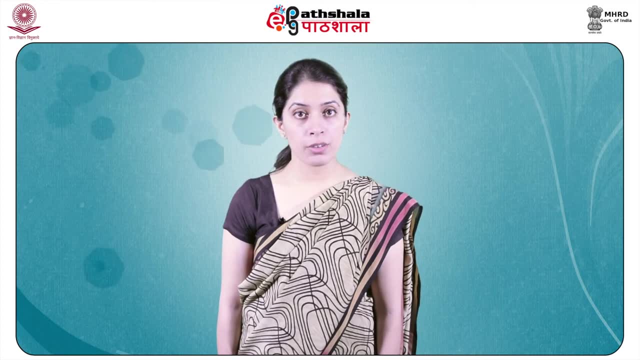 decomposition of this complex to products must be available through translational or vibrational energy of the reactants. Now having a brief introduction to how things occur at the molecular level, Now let us go back to the previous slide. So let us go back to the previous slide, So. 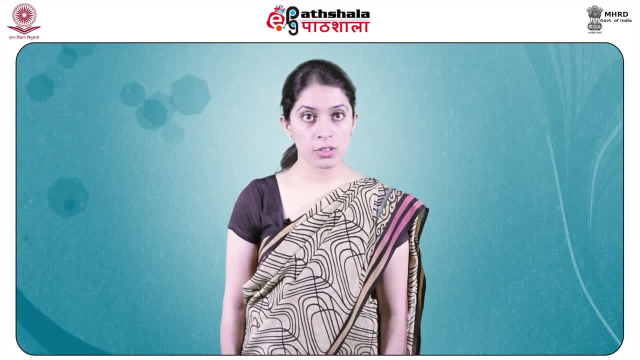 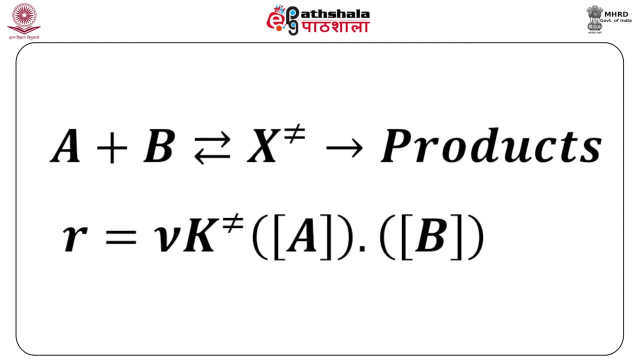 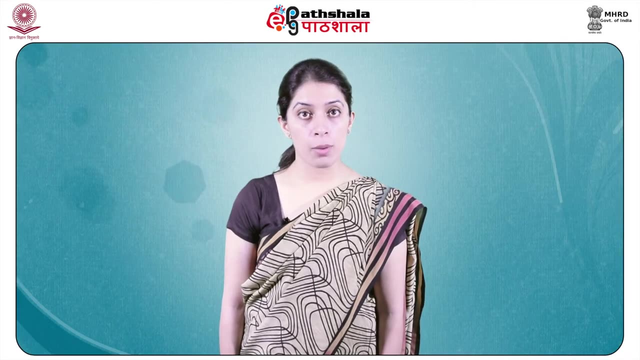 the rate constant equation For the equation as discussed, A plus B, giving transition state complex which gives the products we expressed the rate as frequency into K, into concentration A, into concentration B. Now, since the transition state complex is in a process of decomposition, 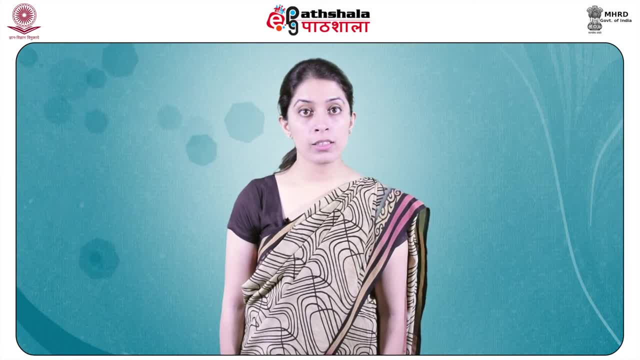 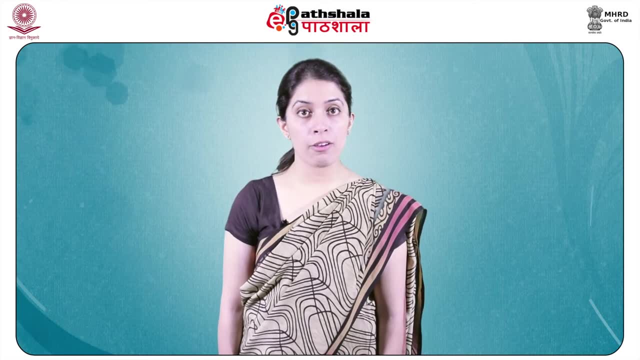 one of its vibrational degree of freedom is in the process of becoming a translational degree of freedom. So let us say E is the rate constant equation. So let us say E is the rate constant equation. So let us say K is the rate constant equation. So let us say K is the rate constant. 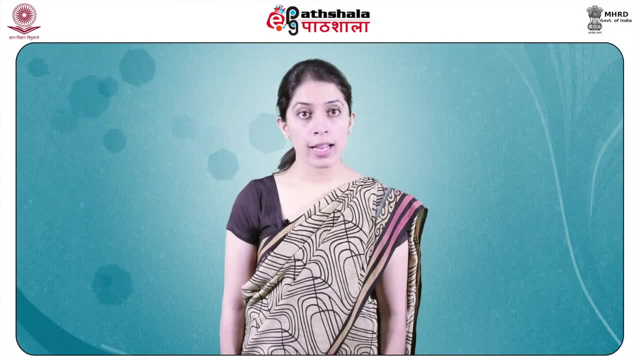 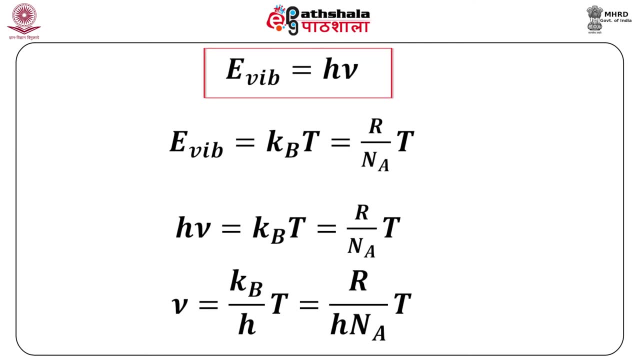 equation. Now, in this case, E can be the average vibrational energy that leads to bond rupturing and, as per the Planck equation for the quantum of energy, E vibration can be expressed as product of Planck's constant and vibrational frequency. 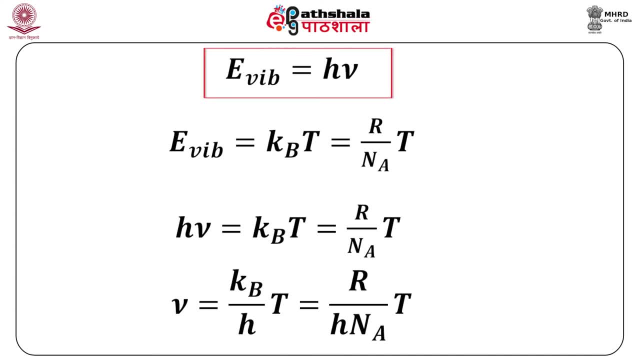 Where H is the Planck's constant and the other term is frequency, and in transition state theory this frequency is taken as the frequency of decomposition of activated complex. As per the classical approach. classical vibration with the transition state function is taking the action of the plant in a process of decomposition of the activated complex In the early days. 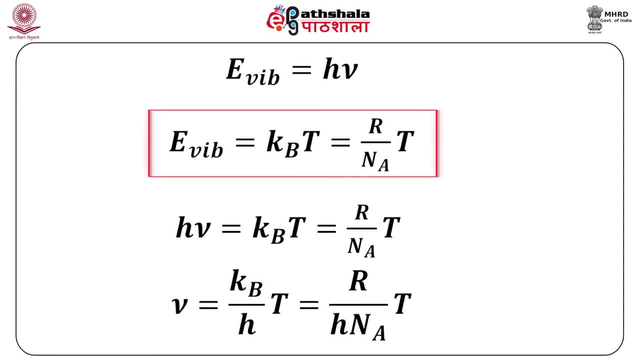 classical vibrational energy is given by the expression E. vibrational equals to KBT, which further becomes equals to R by NA into T, where KB is Boltzmann constant, R is gas constant and NA is the Avogadro's number. Now, equating this energy expression obtained classically with the quantum equation given: 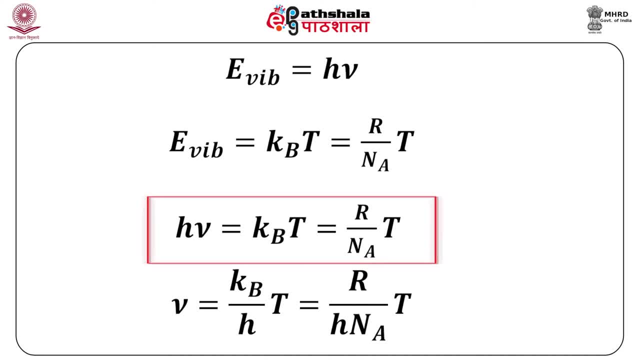 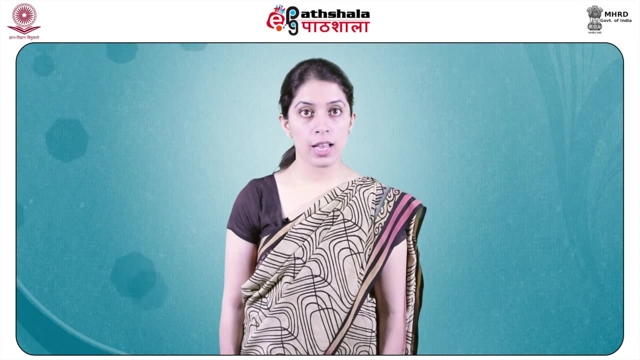 by Planck we get h nu equals to KBT, equals to R by NA T. From this we get the frequency equal to R by h NA into T. Now, substituting this frequency back into the rate expression gives the rate as R upon h NA into T, into K, into concentration, A, into concentration. 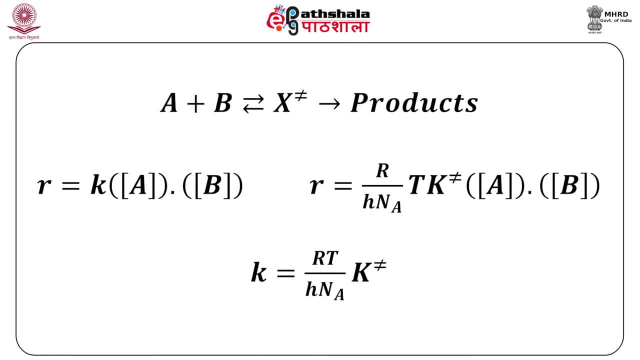 B. Now for the same reaction, A plus B, giving transition state complex, giving product. the classical rate expression is: R equals to K, equals to concentration A into concentration B. Now, on comparing the rate expression obtained from transition state theory and classical approach, we get the value of rate constant K as RT upon h, NA into K. 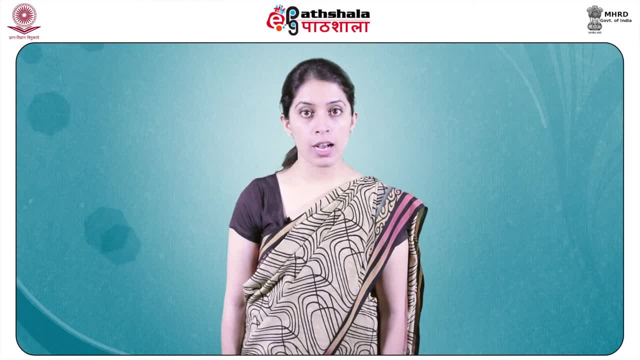 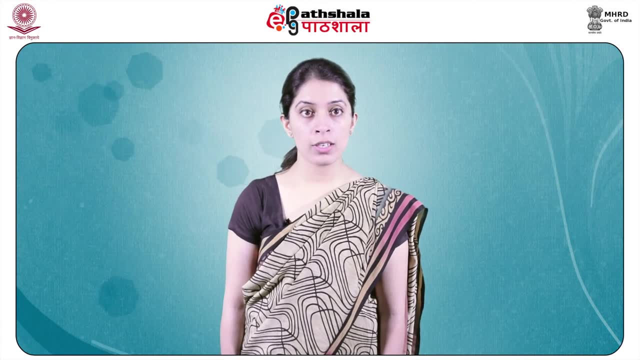 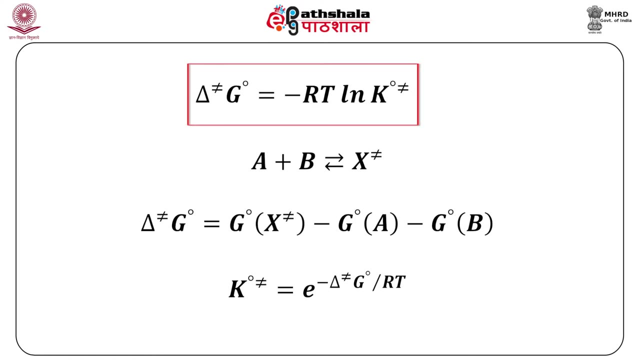 From classical thermodynamics we know that for a reaction occurring at equilibrium Gibbs, free energy And equilibrium constant are related to each other. as per the equation, delta G0 equals to minus RT ln K, where delta G refers to the change in Gibbs free energy and K refers to 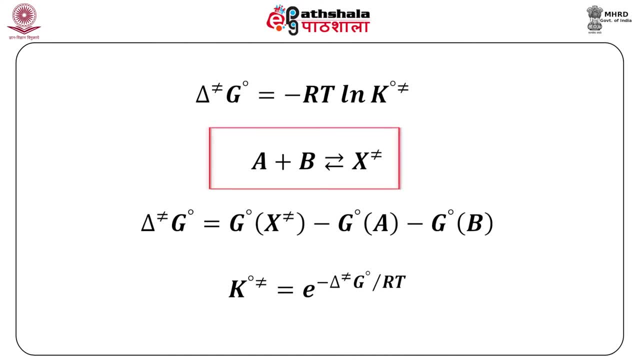 the equilibrium constant. Now, if we consider the reaction A plus B in equilibrium with transition state complex, we get delta G0 as G for transition state complex, minus G for reactant A, minus G for reactant B. Now, rearranging the thermodynamic relation that we have for delta G and K, we get the 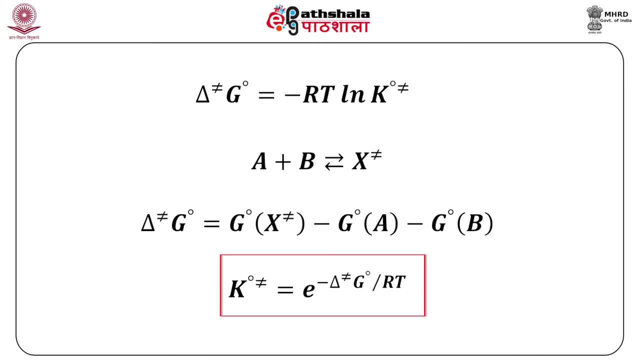 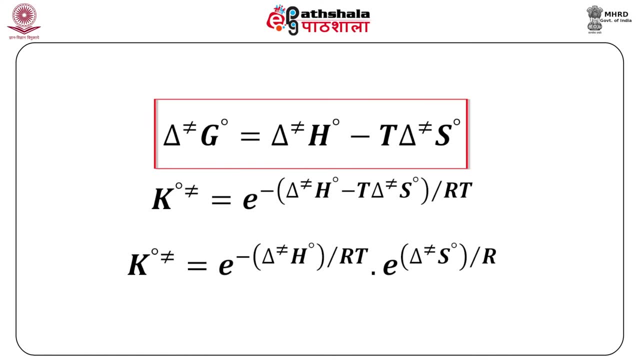 value for equilibrium constant K as e to the power minus GA by RT. Now, as we know from classical thermodynamics, that delta G equals to delta H minus T, delta S, where delta H is the enthalpy change and delta S refers to the entropy change under. 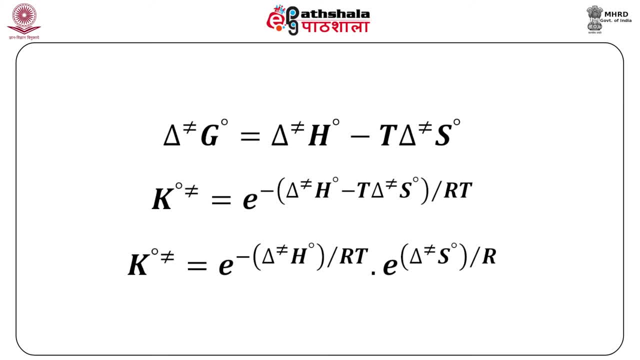 standard conditions. Now, substituting this delta G expression into the equilibrium constant, we get the value of k equal to E to the power minus GA by RT. Now substituting this delta G expression into the equilibrium constant, we get the value of expression. we get equilibrium constant. K0 equals to e to the power minus within brackets. 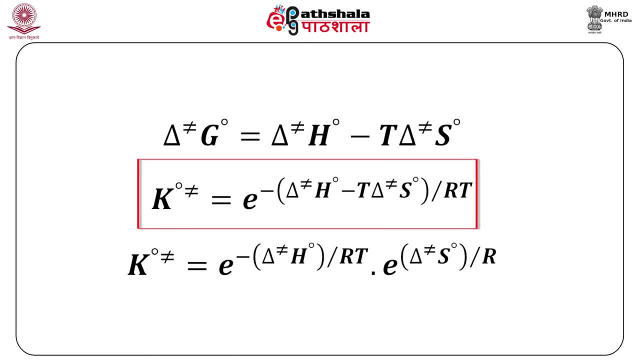 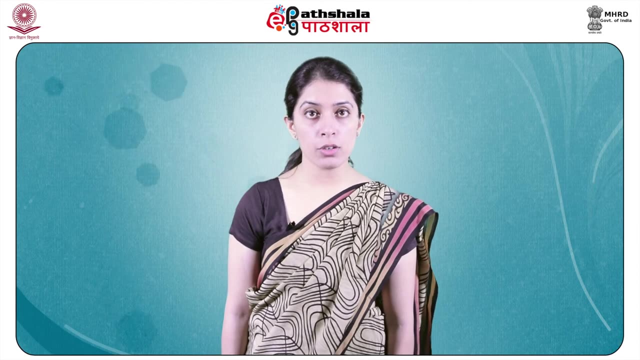 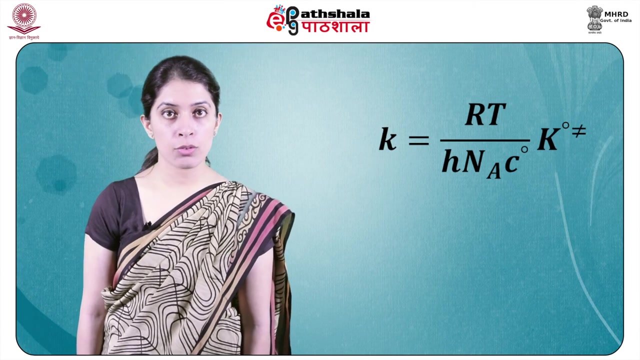 delta H minus T, delta S upon RT. This further simplifies to the expression: K0 equals to e, to the power minus delta H0 upon RT into e to the power delta S0 upon R. Now substituting this into the rate constant expression gives rate constant as K equals to RT upon NA into. 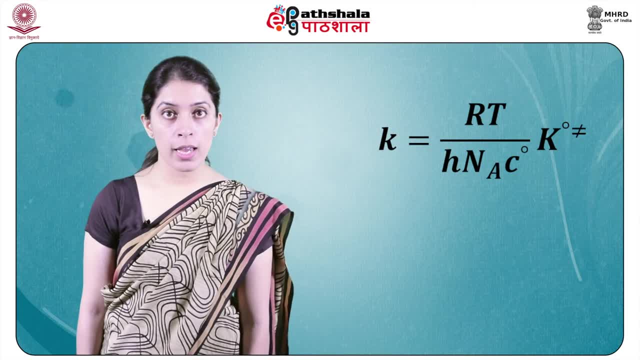 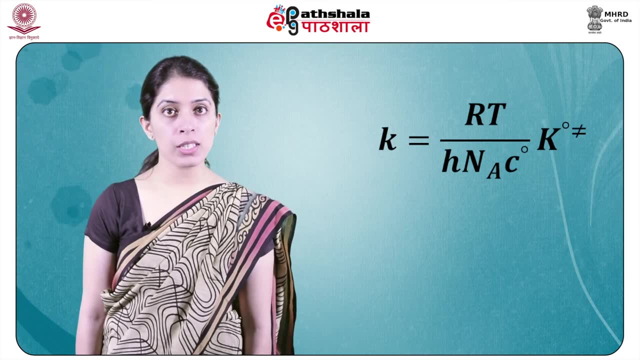 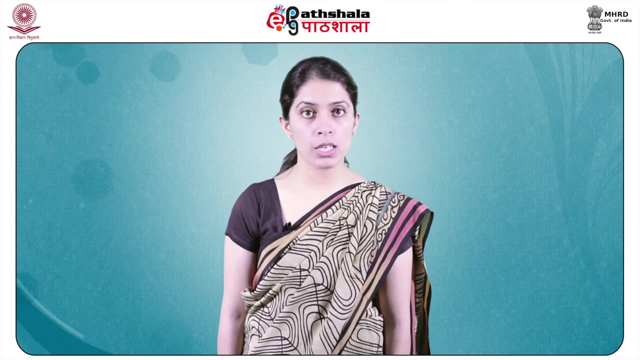 H into C0, into K. Over here it is important to remember that we are throughout using small K for rate constant and capital K for equilibrium constant, Now substituting in this rate constant expression the expression that we have obtained for equilibrium constant in terms of thermodynamic. 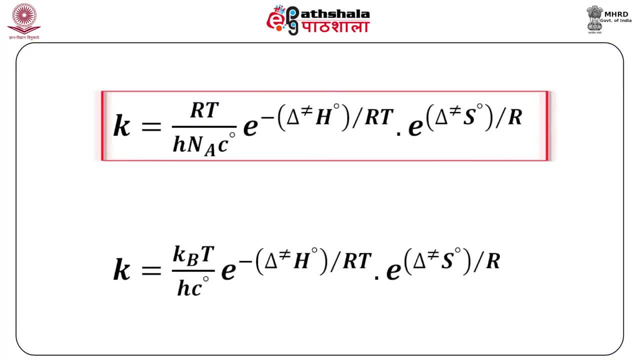 constant Properties. we get rate constant as K equals to RT upon H NA C0 into e to the power minus delta H0 upon RT into e to the power delta S0 upon R. Further simplifying this equation, we get: K equals to KBT upon H C0 into e to the power minus delta H upon RT into e to. 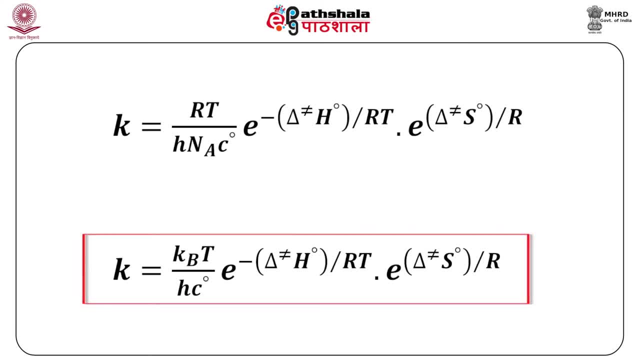 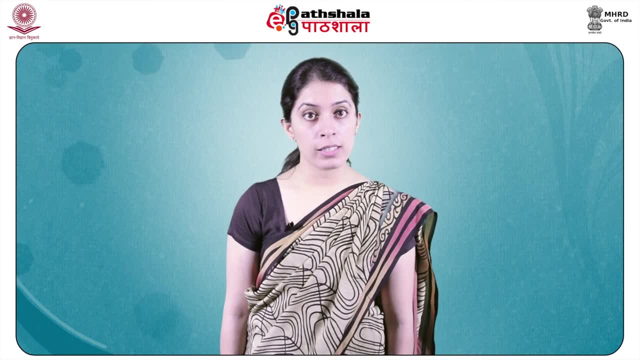 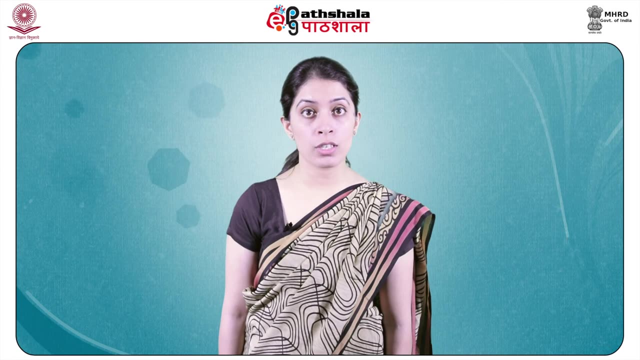 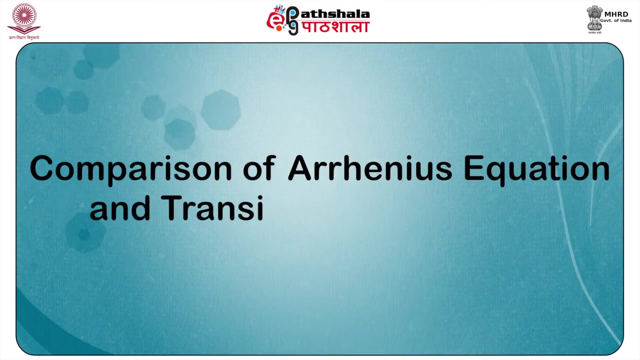 the power delta S0 upon R. This equation is referred to As I ring equation and throughout our discussions over here we have considered only gas phase reactions. The study of these reactions, or reaction rates in solution, is complicated due to the role of solvent, which we will take up in our subsequent modules. Let us now compare the rate constant. 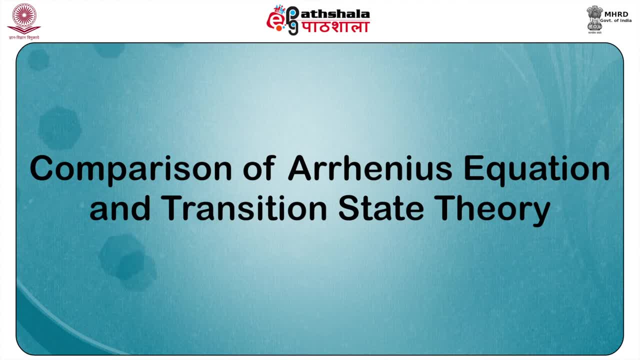 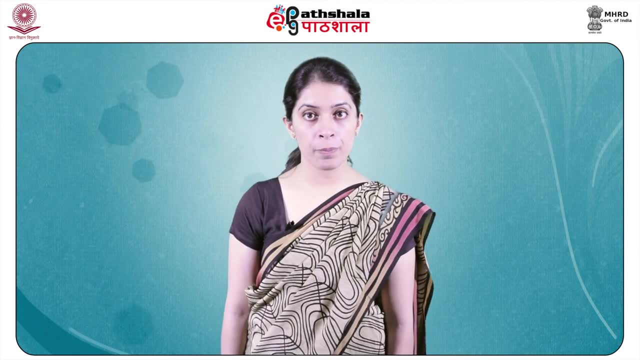 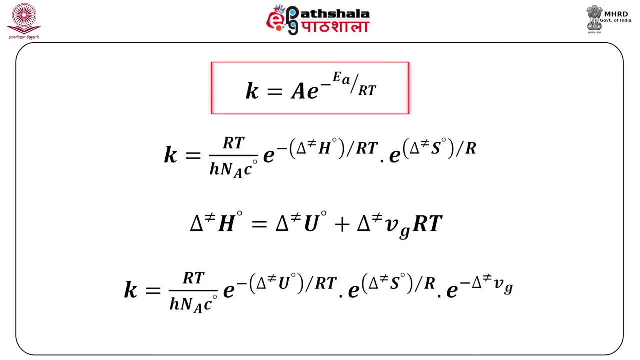 expression that we have obtained from transition state theory with that of Arrhenius equation. We did discuss in detail the Arrhenius equation in our earlier module, where we saw that rate constant is expressed in the following manner: k equals to a into e, to the power minus e, a by r, t and as per transition state theory we obtained 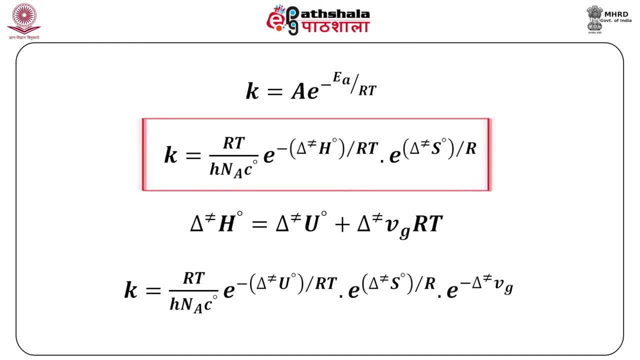 the rate constant as r t upon h. na c naught into e to the power minus delta h naught upon r t into e to the power delta s naught upon r. Now for gaseous systems, we know that delta h can be expressed thermodynamically in the manner: delta h naught equals to delta u naught, plus change in. 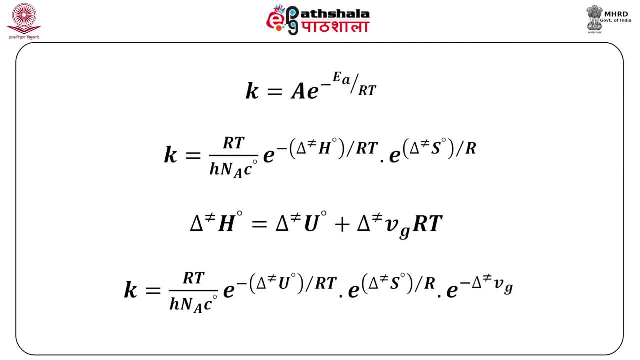 number of moles into r, into t. Now, substituting this delta h value in the rate constant expression gives us k equals to r t upon h into na, into c naught into e to the power minus delta u naught upon r t into e to the power delta s naught upon r. 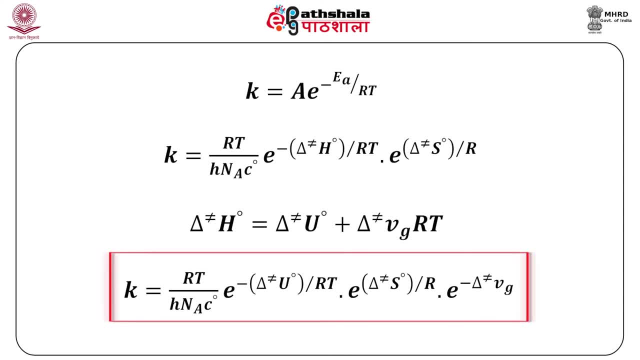 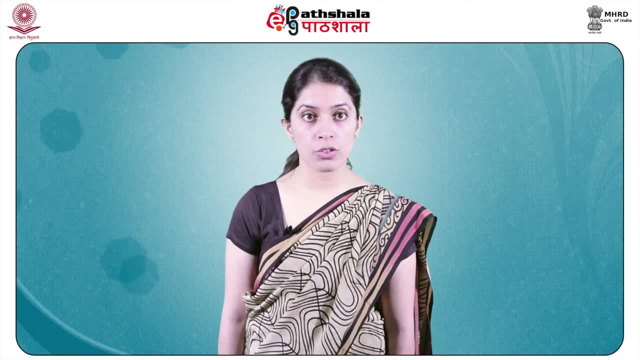 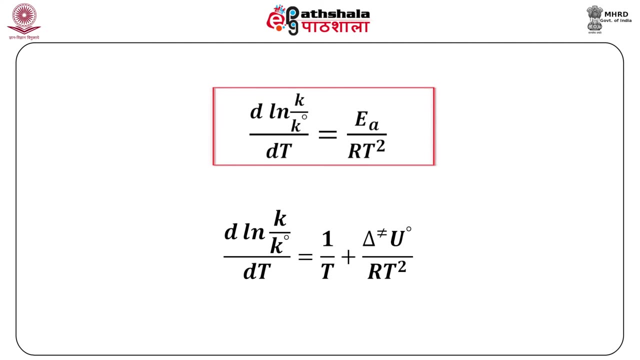 into e to the power minus change in number of moles. Taking logarithm of these equations and differentiating them with respect to temperature, from Arrhenius equation we get the expression as d, ln, k by k. naught upon dt equals to e. a upon r t square. 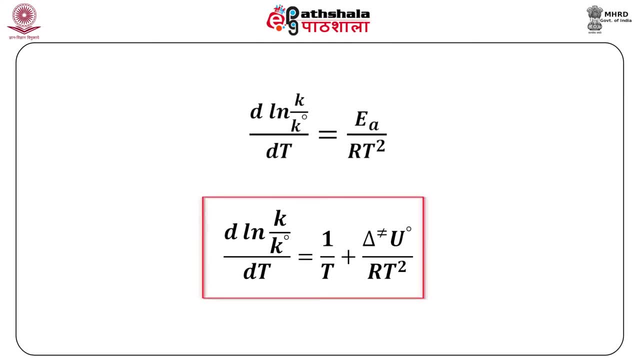 And from transition state theory we get the expression as d ln, k by k. naught upon dt equals to 1 upon t plus delta u naught upon r t square. On comparing the two, we get the expression as: e. a upon r t square equals to 1 upon t plus delta u naught upon r t square. Now, from this we get: 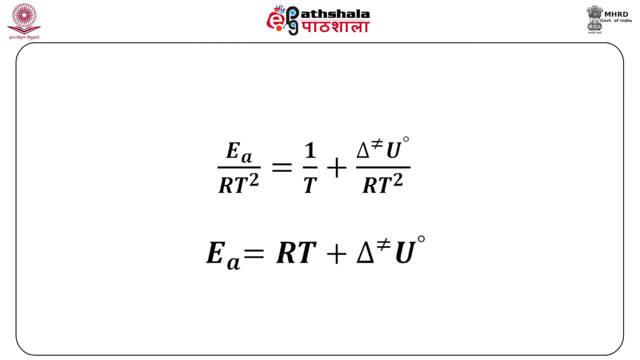 the relation between activation energy and the energy obtained from transition state theory, and the expression that we obtain is of the form e, a equals to r, t plus delta, u naught, And from thermodynamics we know that h is equals to u plus p v. So at constant pressure, 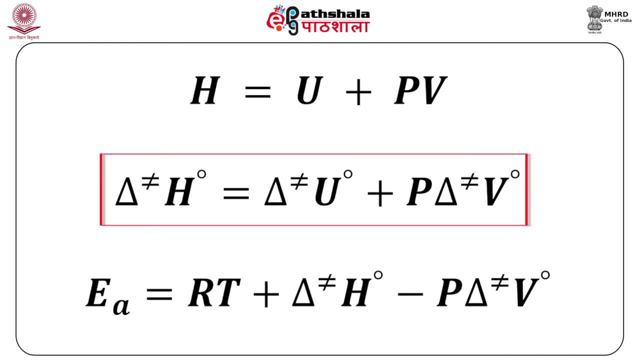 we get the expression as delta h naught equals to delta u naught plus p delta v naught. So e a becomes equals to r t plus delta h naught minus p delta v naught. Now this equation that we have obtained can be applied to both condensed phase and gas phase reactions. 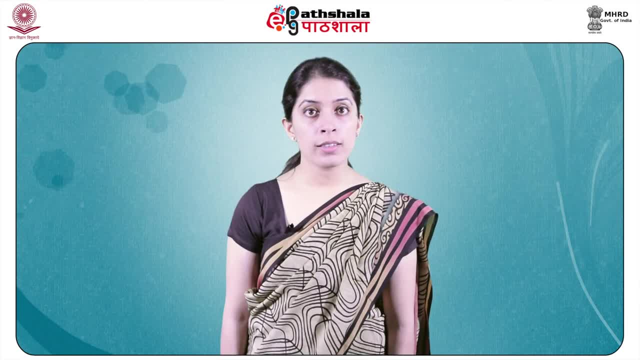 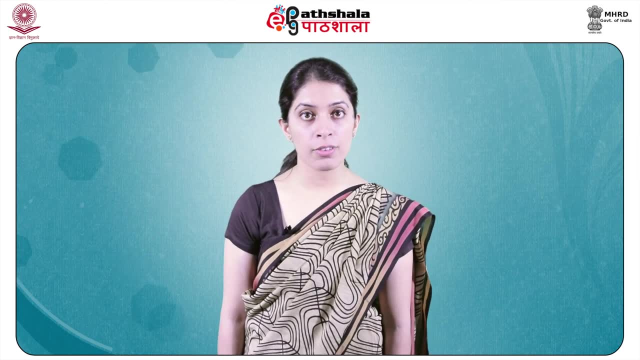 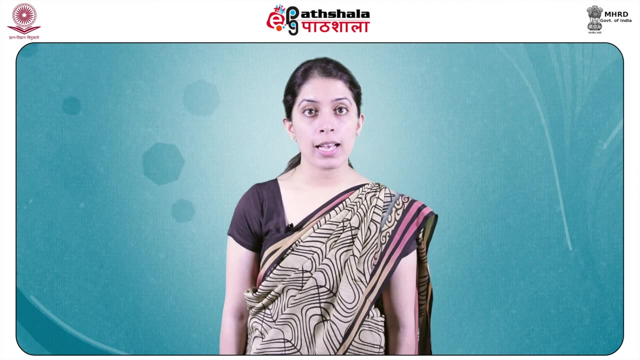 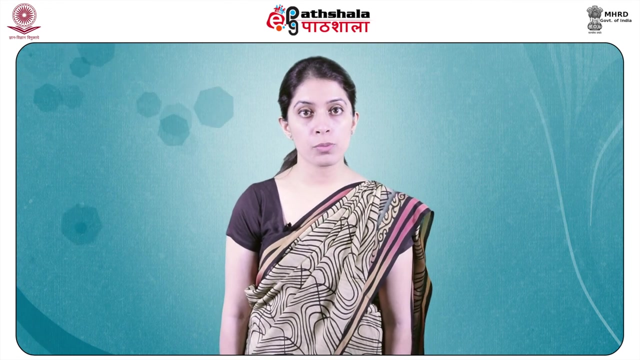 In all. in this module we studied transition state theory. This transition state theory was developed in 1935 and this depicts the formation of transition state complex from reactants A and B as a proceeding step for the formation of products. This theory essentially assumed that the collisions are responsible for a chemical reaction and equilibrium exists. 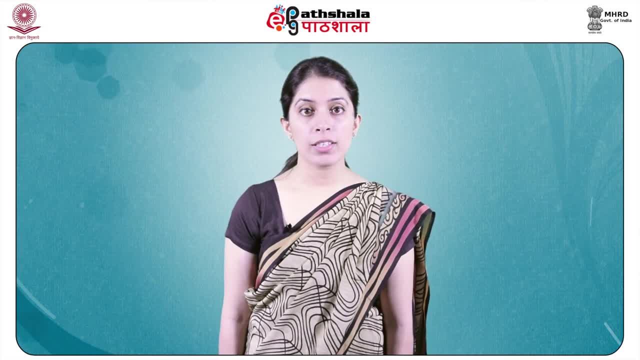 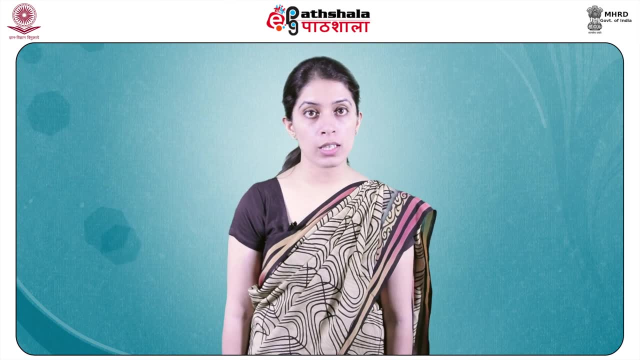 between the reactants and the transition states. So this is what we are going to do in the next session: transition state complex and the reaction coordinate describing the conversion of transition state complex to product can be mapped out on a single degree of freedom of transition.